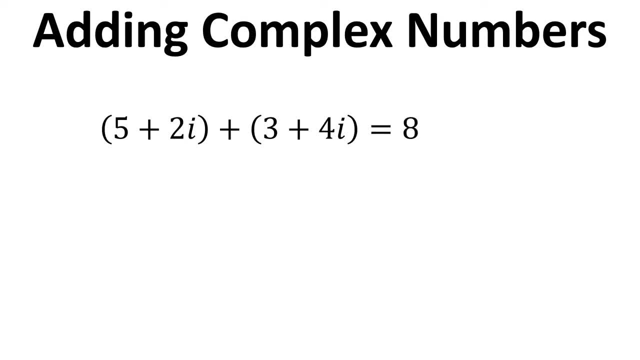 imagine. it's a very complex number. It's a very complex number and it's a very straightforward. We just add up the real component, so 5 plus 3 gives us 8. and then we add up the imaginary numbers, so 2i plus 4i gives us 6i. Okay, what about? 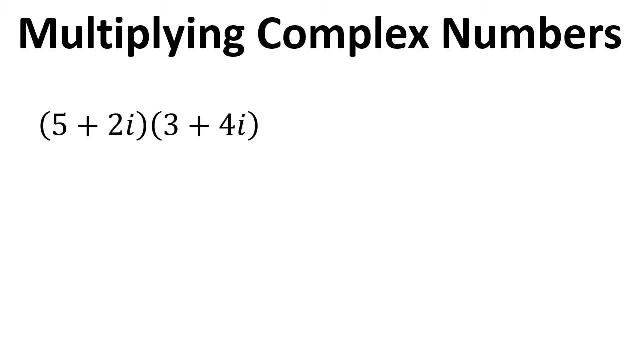 multiplying complex numbers. So here's another example: we've got 5 plus 2i multiplied by 3 plus 4i. So to start with, we multiply the two real numbers, that gives us 15.. Then we multiply the real numbers by 3, and then we multiply the. 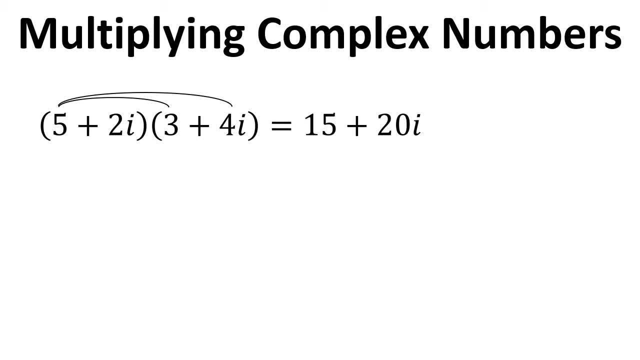 real number from the first complex number with the imaginary number from the second complex number. that gives us 20i. Then we do the same thing, but it's the other way around. now We've got the imaginary number times the real number and then we multiply the two imaginary numbers and that gives us 8i squared. 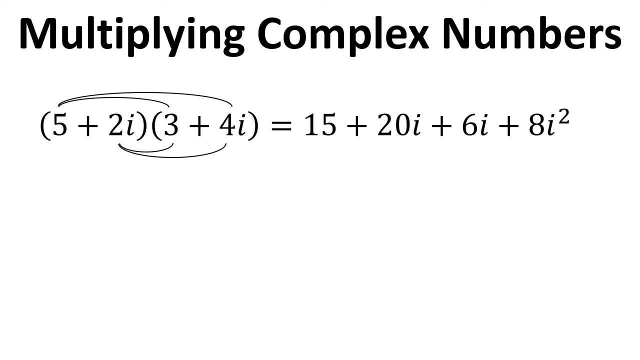 Okay. so now we need to simplify this. So we still have 15, but we can add the 20i and the 6i to give us 26i. So now we need to simplify this. so we still have 15, but we can add the 20i and the 6i to give us 26i. 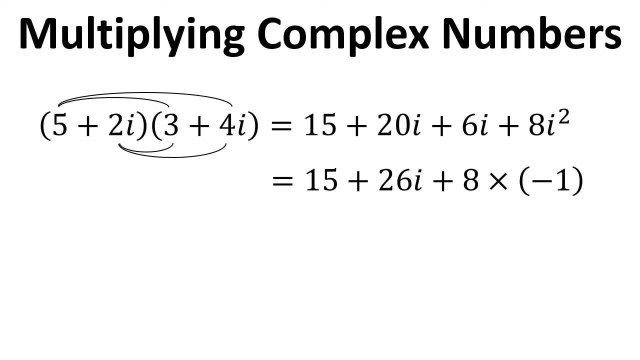 and i squared is minus 1, so 8 times minus 1 is minus 8, and so the overall number there then is 7 plus 26i, because we need to do the 8 and we need to do the 15. take away the 8.. Okay, final thing I want to mention, then, is that 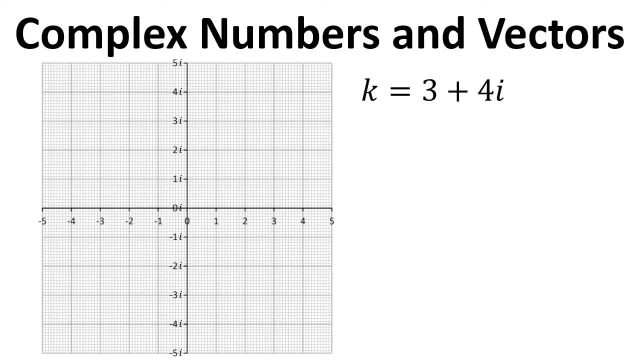 complex numbers can be represented as vectors. So if we have vector K equals 3i plus 4i- sorry, 3 plus 4i. we can plot that out on a graph where we have the real number line on the x-axis. 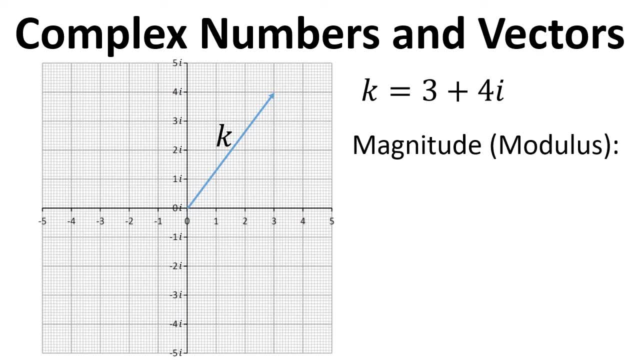 and the imaginary number line on the y-axis, and we can also get the magnitude of the vector, or it's also referred to as the modulus, and the symbol for that is the k to represent the vector, and then these two vertical lines, and we just work it out using Pythagoras.